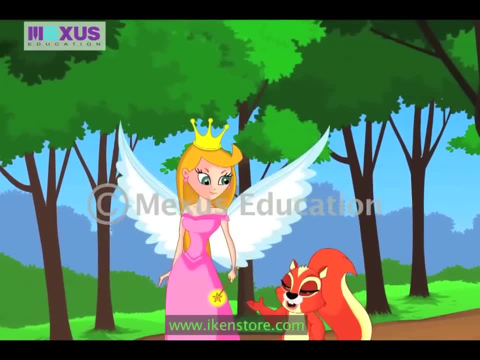 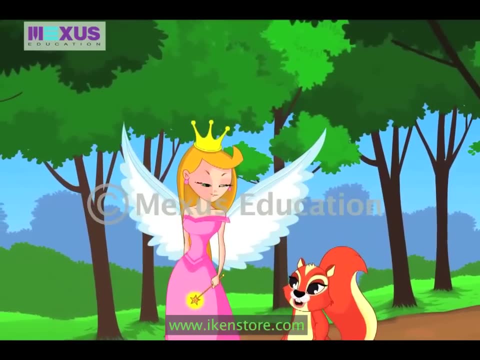 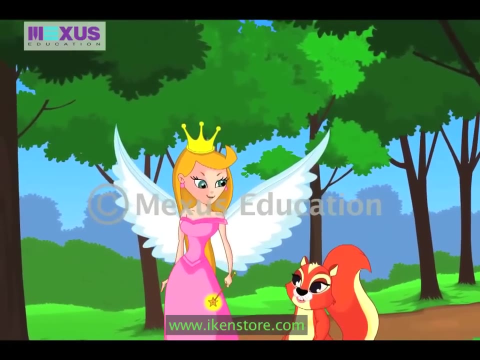 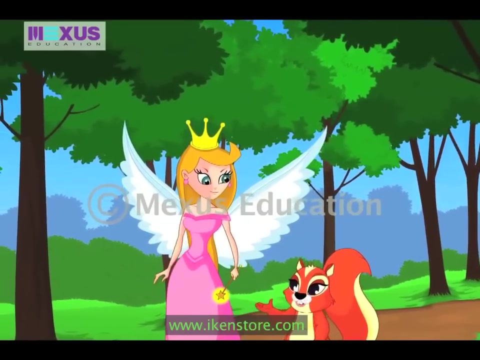 Okay, Tell me what is 2 multiplied by 4? 8? That was easy. What is 8 multiplied by 7? 56? Okay, okay. What is 9 multiplied by 9? 81? Alright, you win. Now will you tell me how do you solve the problems so quickly? 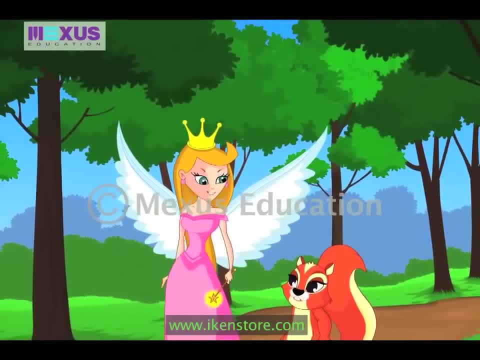 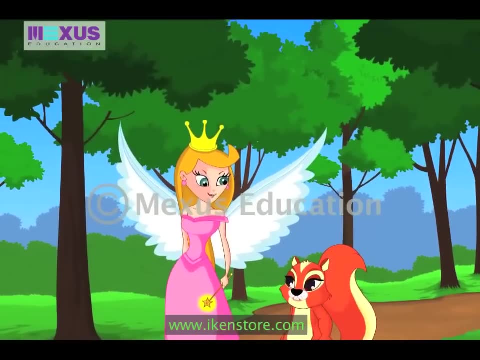 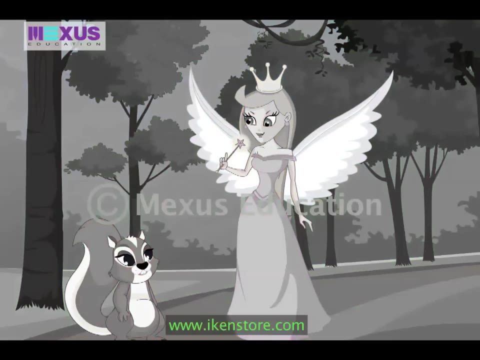 Actually, it is a very nice trick that I have found out. Teach me this wonderful trick, fairy, Please. Alright, The trick is learning the multiplication tables. Basically, a multiplication table for a number is a list obtained by multiplying the number with other numbers. 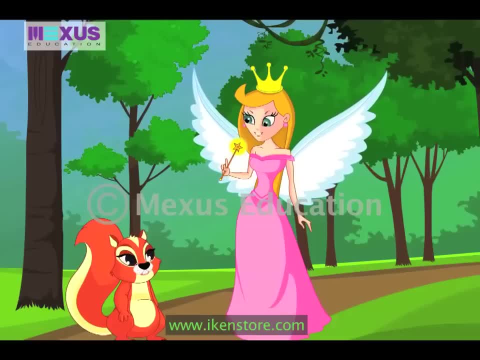 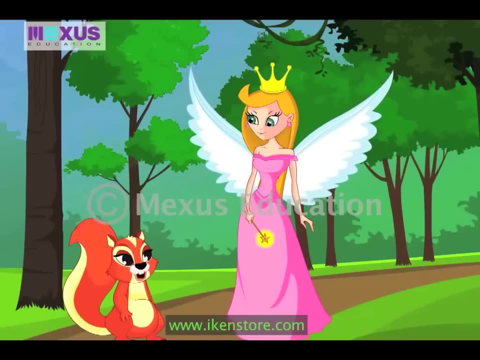 Once you memorize these tables, multiplication will be on your finger tips. Sounds good. I want to learn these multiplication tables, These multiplication tables, too. Sure, Amber. Let's start with the multiplication table of number 1.. 1 ones are 1.. 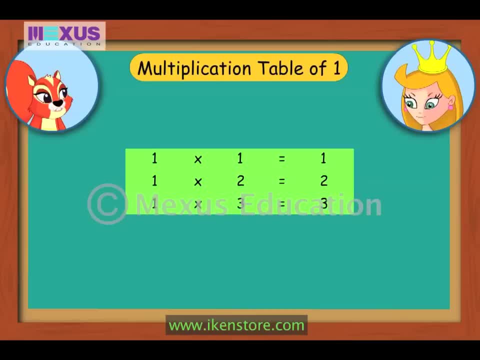 1. twos are 2.. 1. threes are 3.. 1. fours are 4.. 1. fives are 5.. 1. sixes are 6.. 1. sevens are 7.. 1. eights are 8.. 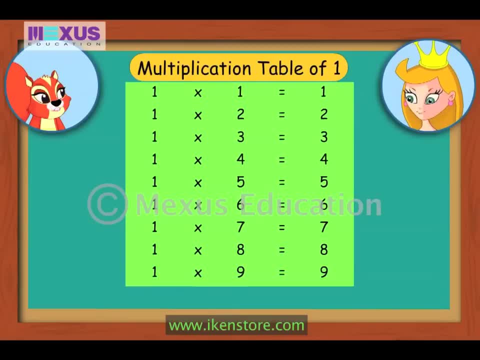 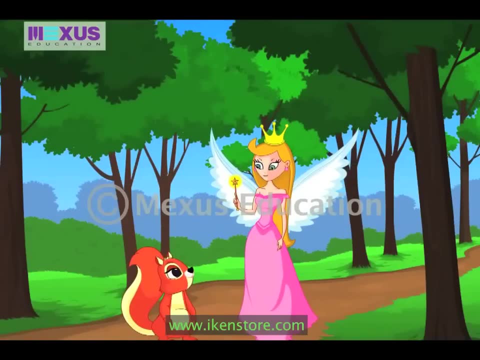 1 nines are 9.. 1 tens are 10.. That is the multiplication table of 1.. Now we shall go on to the multiplication table of 2.. 2 ones are 2.. 2 twos are 4.. 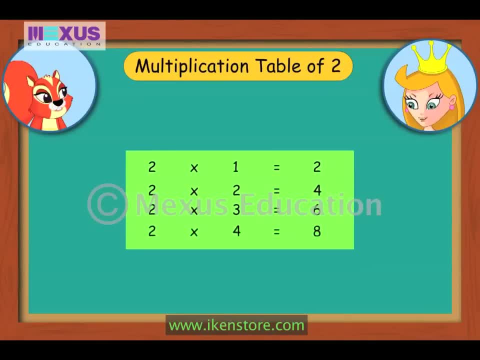 2 threes are 6.. 2 fours are 8.. 2 fives are 10.. 2 sixes are 12.. 2 sevens are 14.. 2 eights are 16.. 2 nines are 18.. 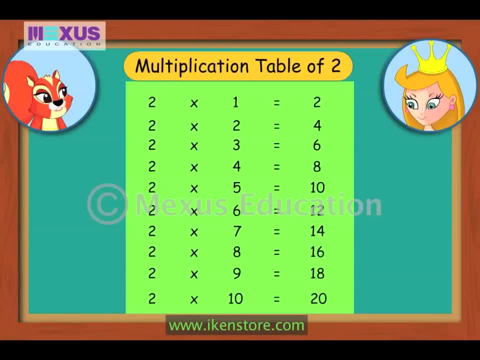 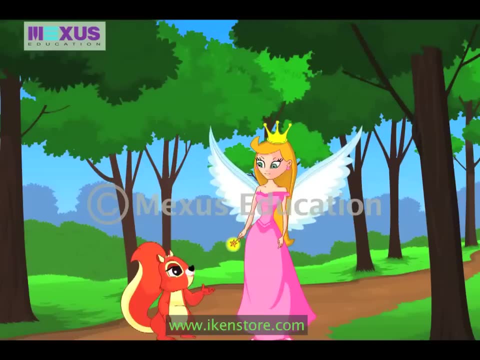 2 tens are 20.. Isn't that easy, Amber. Yes, Fairy, I will only have to learn them Now. next table is going to be of the number 3,, right, Correct. Let us begin with the 3 times table. 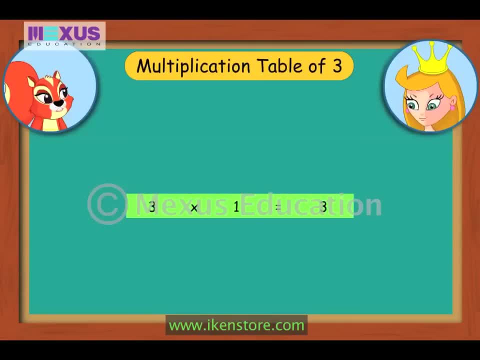 3 ones are 3.. 3 twos are 6.. 3 threes are 9.. 3 fours are 12.. 3 fives are 15.. 3 sixes are 18.. 3 sevens are 12.. 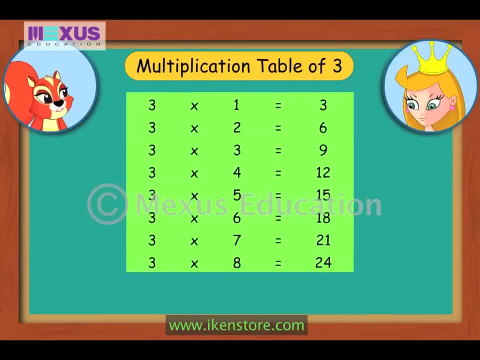 3 sevens are 21.. 3 eights are 24.. 3 nines are 27.. 3 tens are 30.. Now we will move on to the 4 times table. 4 ones are 4.. 4 twos are 8.. 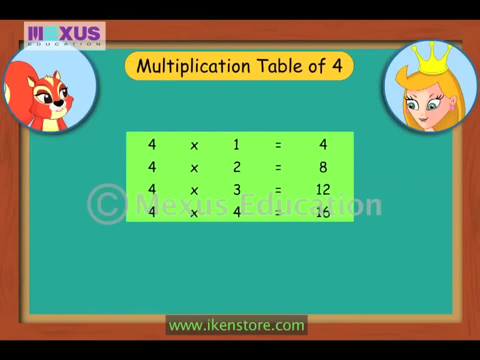 4 threes are 12.. 4 fours are 16.. 4 fives are 20.. 4 sixes are 24.. 4 sevens are 28.. 4 eights are 32.. 4 nines are 36.. 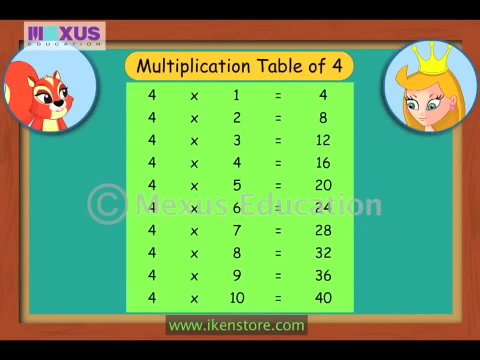 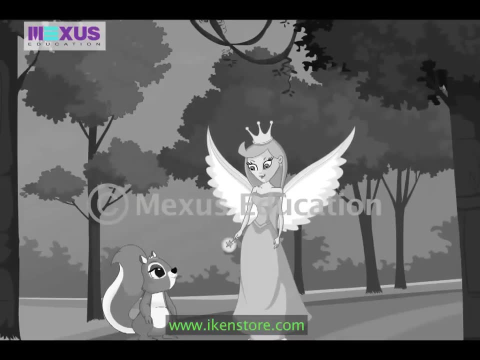 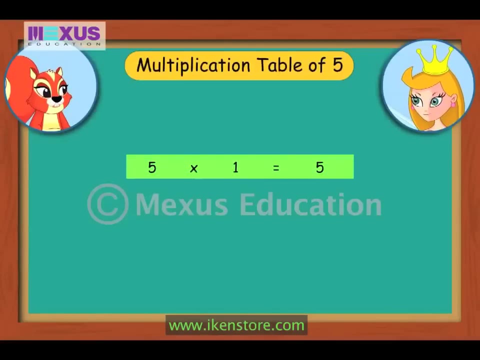 4 tens are 40.. Did you get that Amber? Yes, Fairy. So are you ready for the next one? Next is the multiplication table. 5 ones are 5.. 5 twos are 10.. 5 threes are 15.. 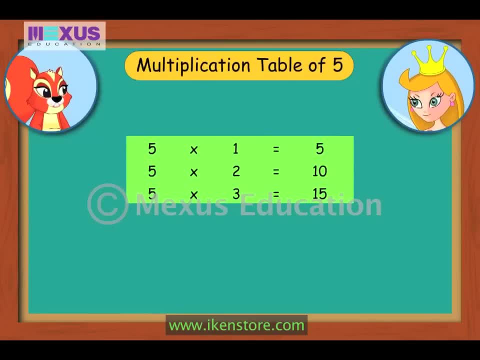 5 fours are 20.. 5 fives are 25.. 5 sixes are 30.. 5 sevens are 35.. 5 eights are 40.. 5 nines are 45.. 5 twos are 40.. 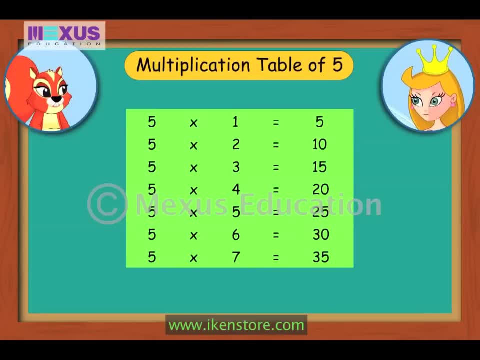 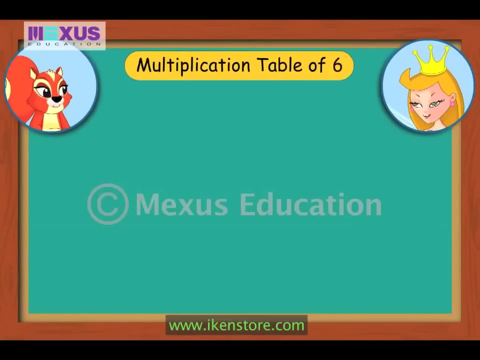 5 sixes are 35.. 5 eights are 40.. 5 nines are 45.. 5 twos are 40.. 5 sixes are 45.. 5 tens are 50.. Now let us see the multiplication table of 6.. 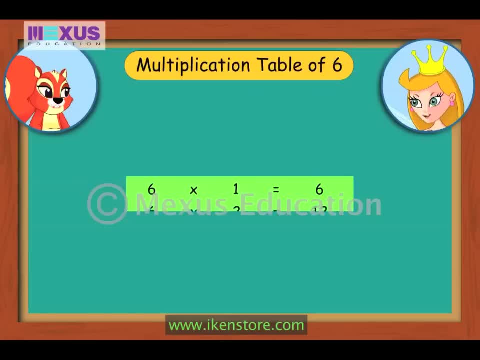 6 ones are 6.. 6 twos are 12.. 6 threes are 18.. 6 fours are 24.. 6 fives are 30.. 6 sixes are 36.. 6 sevens are 42.. 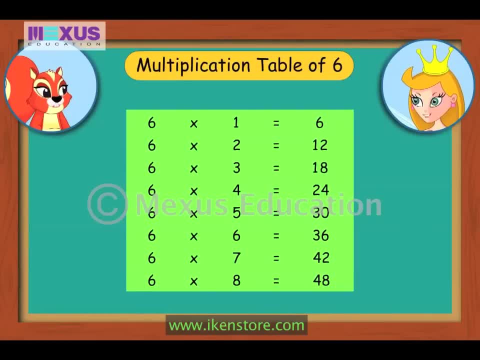 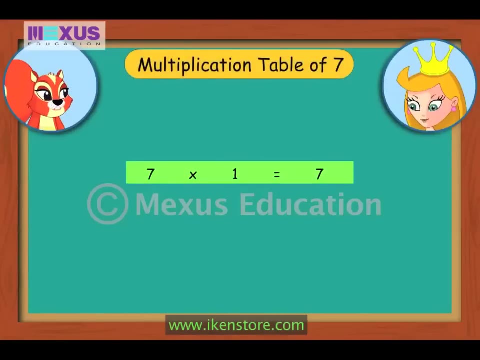 6 eights are 48.. 6 nines are 54.. 6 tens are 60.. Now for the multiplication table of 7.. 7 ones are 7.. 7 twos are 14.. 7 threes are 21.. 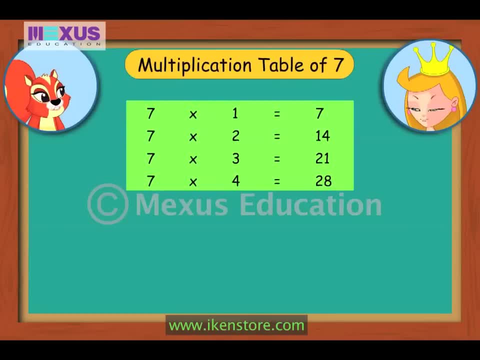 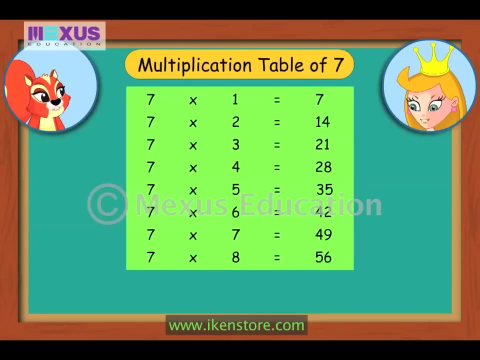 7 fours are 28.. 7 fives are 35.. 7 sixes are 42.. 7 sevens are 49.. 7 eights are 56.. 7 nines are 63.. 7 tens are 70.. 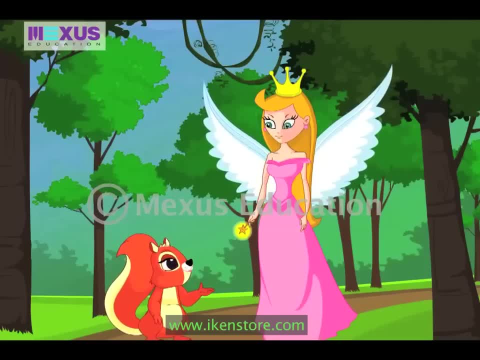 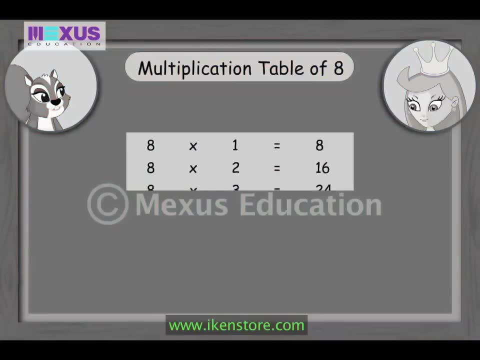 Time for the multiplication table of 8.. 8 ones are 8.. 8 twos are 16.. 8 threes are 24.. 8 fours are 32.. 8 fives are 40.. 8 sixes are 48.. 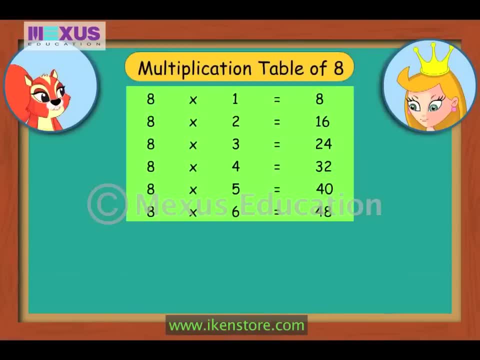 8 sevens are 56.. 8 eights are 64.. 8 nines are 72.. 8 tens are 80.. All set for the multiplication table of 8.. 8 eights are 64.. 8 nines are 72.. 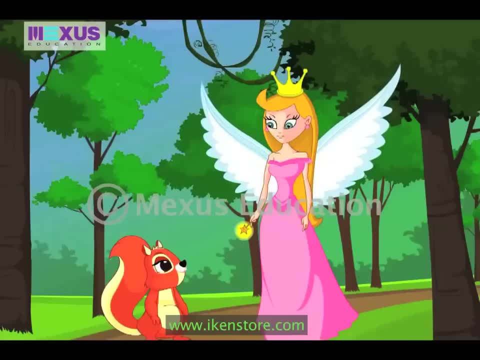 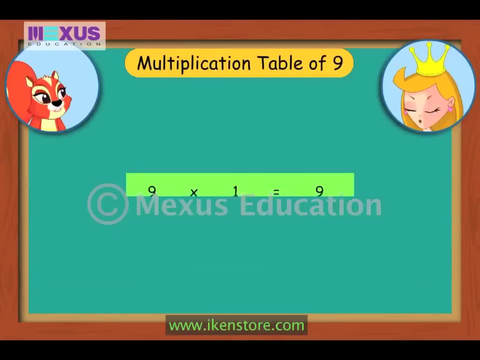 8 tens are 80.. All set for the multiplication table of 8.. All set for the multiplication table of 9, Amber: Yes, 9 ones are 9.. 9 twos are 18.. 9, threes are 27.. 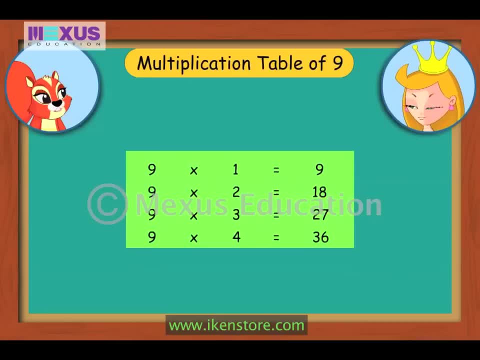 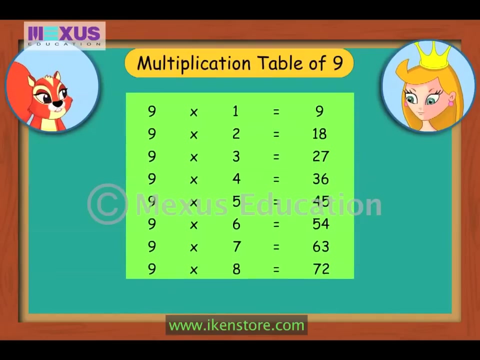 9 fours are 36.. 9 fives are 45.. 9 sixes are 54.. 9 sevens are 63.. 9 eights are 72.. 9 nines are 81.. 9 tens are 90.. 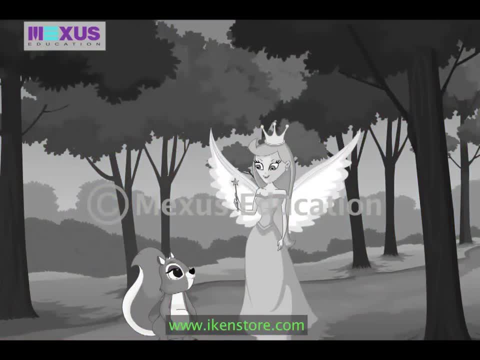 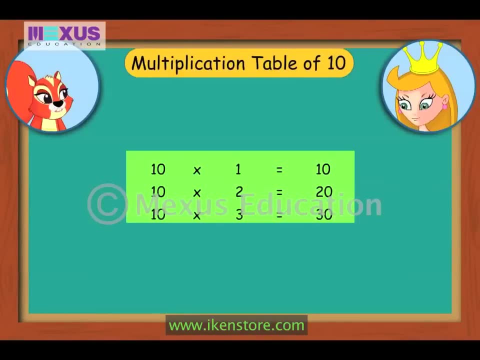 Finally, here is the multiplication table of 10.. 10 ones are 10.. 10 twos are 20.. 10 threes are 30.. 10 fours are 40.. 10 fives are 50.. 10 sixes are 60.. 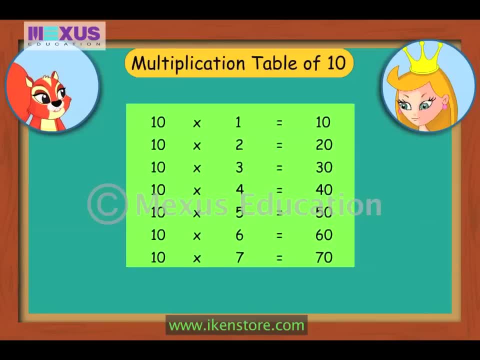 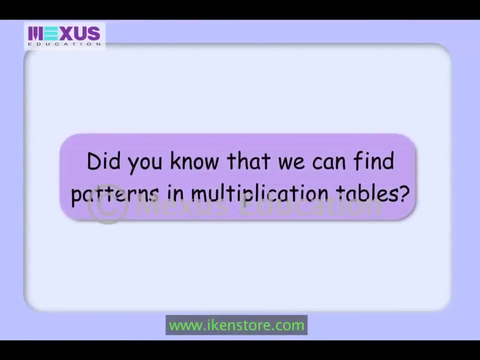 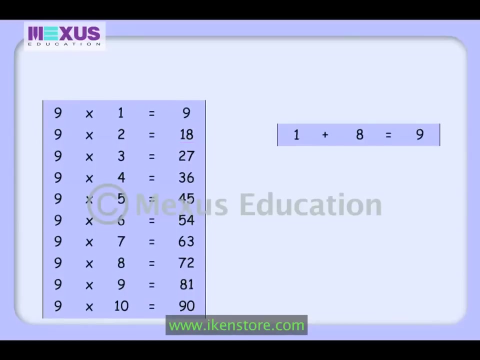 10 sevens are 70.. 10 eights are 80.. 10 nines are 90.. 10 tens are 100.. 10 threes are 150.. 20 twos are 1.. 12 heads are 15.. 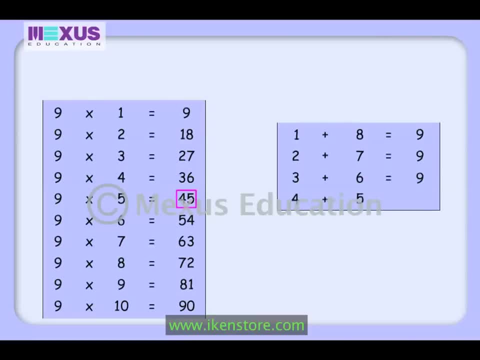 2 girls are 40.. 20 minas are 63.. 6 tutas are 70.. 2 threes are 15.. You must say your scores are correct at one go. Step 1. Carefully алή. delightful day at Atalante Gábor. 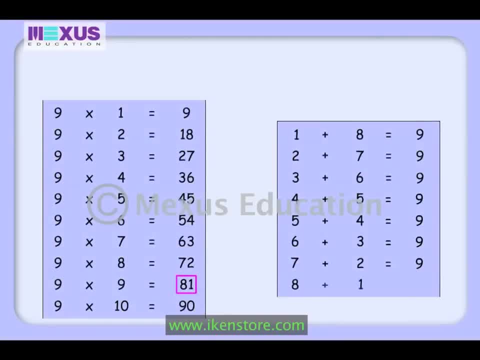 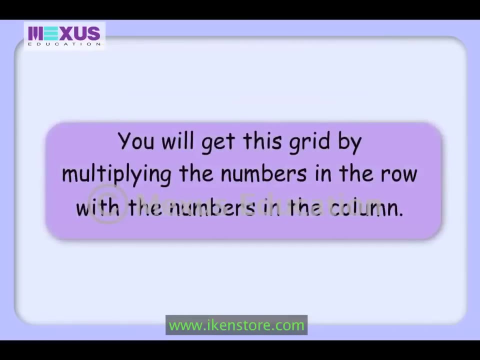 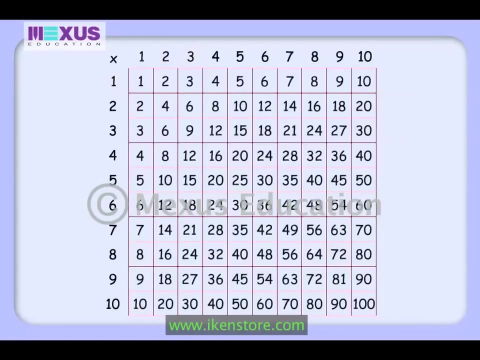 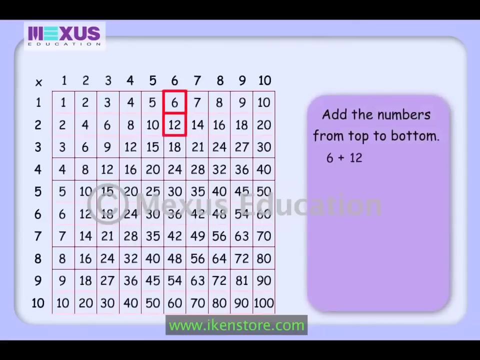 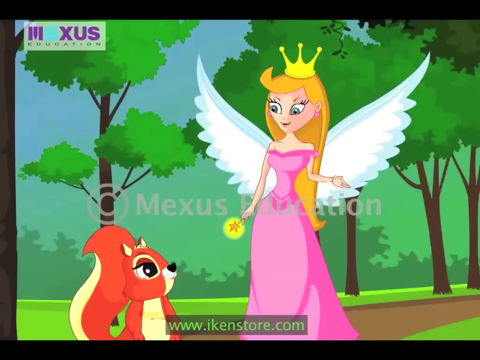 Did you come from Bequia, Thank you. So isn't multiplication interesting? Once you memorize your tables, you can easily solve any multiplication problem. Hey, thanks a lot, Fairy. I will memorize all the multiplication tables. I'll leave now. 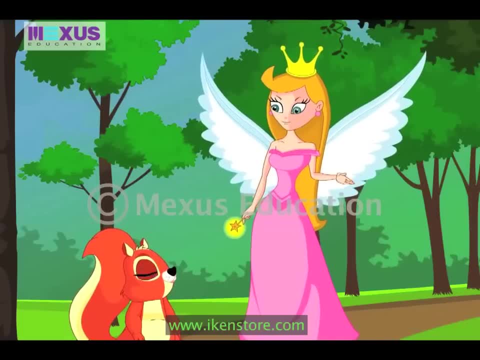 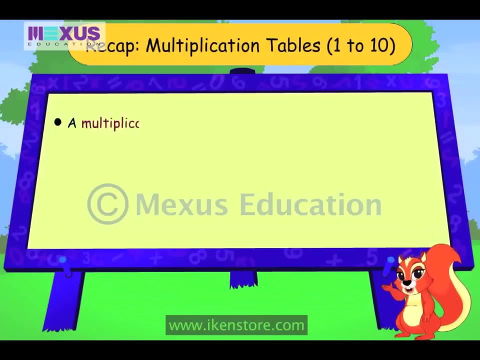 Have to study for tomorrow's test. I am sure it will go well, Amber. bye and all the best. Bye-bye and thanks a lot. Hi friends, Let us quickly recap this lesson. A multiplication table for a number is a list obtained by multiplying the number with other numbers, starting from 1 in ascending order.